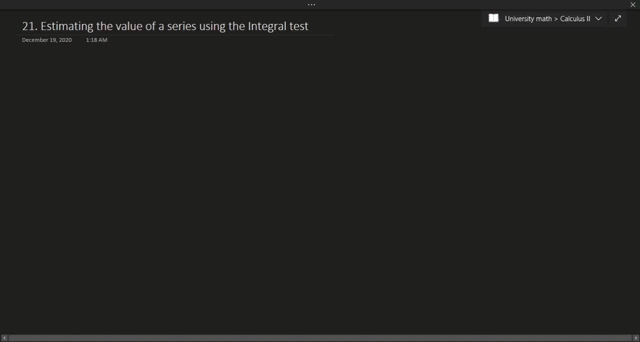 So, as I mentioned, we can use the integral test to find out how accurate a sum is when estimating the value of a series, And that is given by the following kind of inequality: So it turns out that when you sum from N plus 1 to infinity, so the N plus first term in essence of F of X. 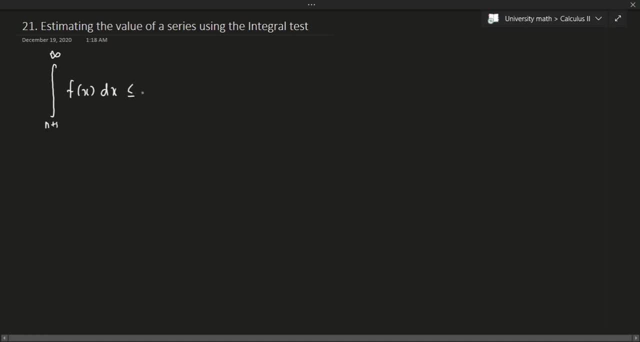 times dx, that's always going to be less than or equal to some remainder, And when I say remainder, the remainder comes from essentially something up from N equals k plus 1 – or let me make this very clear – the remainder comes from the fact that we have Rn is going to be equal to a. 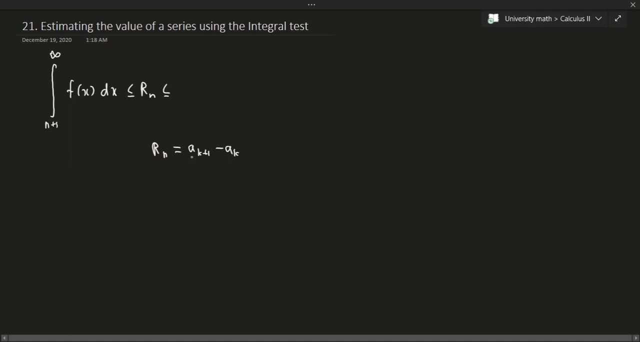 k plus 1 minus ak. So basically the difference in the next term above and the term that originally we're working with. that's going to be the leftover remainder that we have. So it turns out that using the integral test, we have this following inequality: So the integral from n. 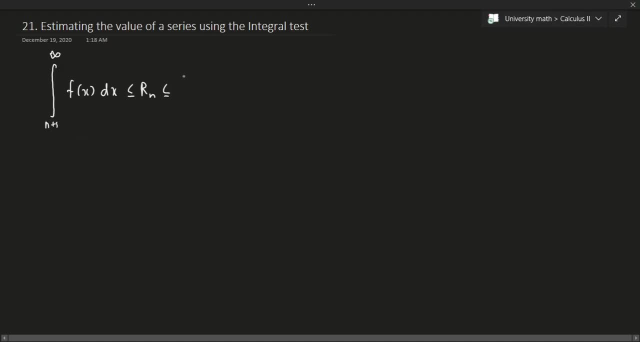 plus 1 to infinity is going to be less than or equal to the remainder, which is less than or equal to the integral from n to infinity, of f of x times dx. So this might seem very absurd and very confusing at first, But what I'm essentially saying is that the remainder is always going to 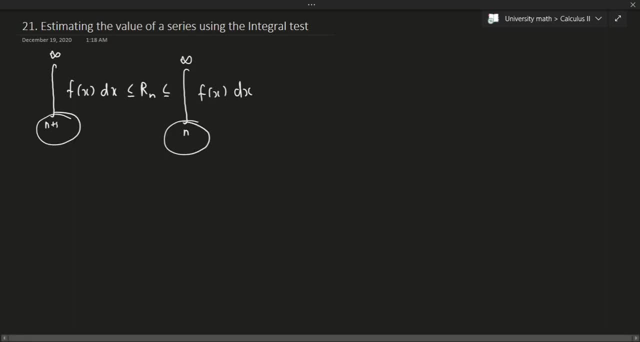 be bounded between the n plus first term and the nth term. More importantly, this is the integral test, essentially. So, basically, whatever error I want or, in this case, the error being the remainder, whatever error I want is always going to be less than or equal to some integral. 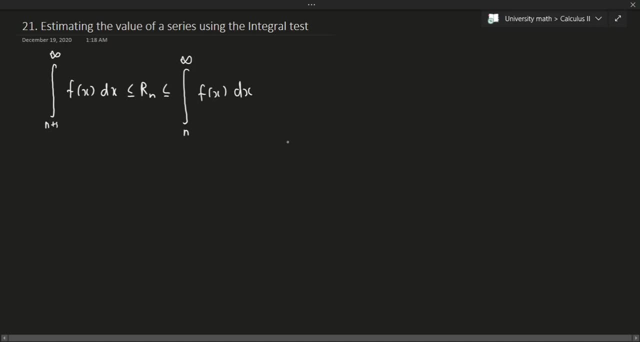 Intuitively, this makes a lot of sense if you think about it As a series is a bunch of discrete points. an integral is a set of continuous points. So if you take a bunch of continuous points and sum them all up, 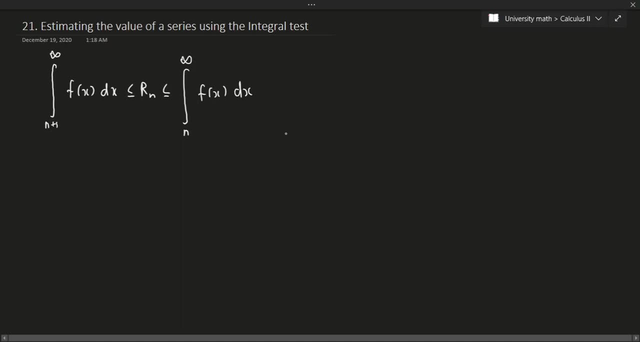 it's always going to be more than a bunch of discrete points, if you think about it, Because in a bunch of discrete points, instead of discrete points, I'm always excluding a few things. I'm excluding this kind of part. I'm excluding this part, this part, this, this, this and this. 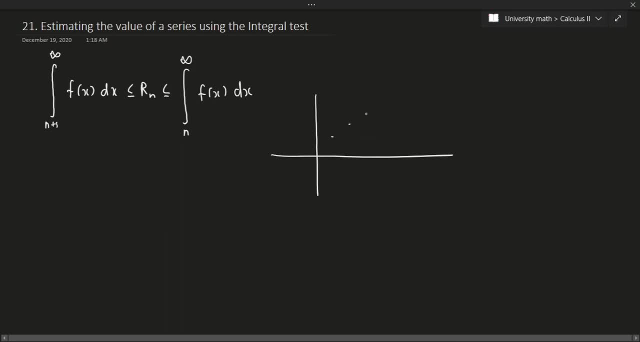 I'm always excluding a few things, So I'm always going to have some gaps in this estimate. But for continuous points I don't have that issue. I'm filling in every single possibility from whatever bounds I'm picking. So as a result, it intuitively should make sense that the integral is going to be a lot more accurate. 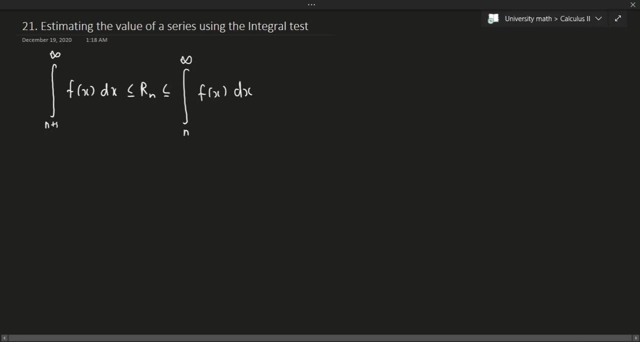 than whatever remainder I have from using series. But how does this actually help us? you know, determine how accurate we need to be in order to make sure our error is less than some threshold. How does this help us? Well, let's go ahead and talk about this with an example. 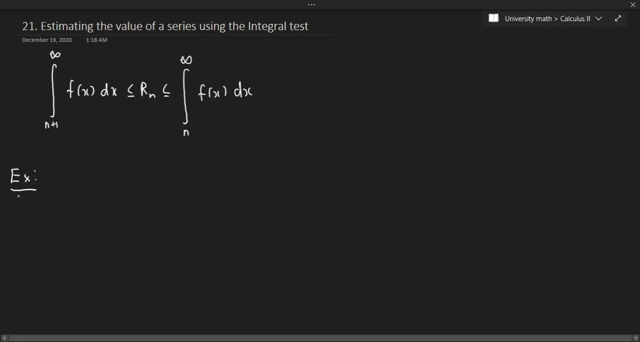 So hopefully this will kind of help us. So example: Okay, So approximate or approximate the summation from n equals 1 to infinity of 1 over n, n squared using the first 10 terms, and estimate the error. 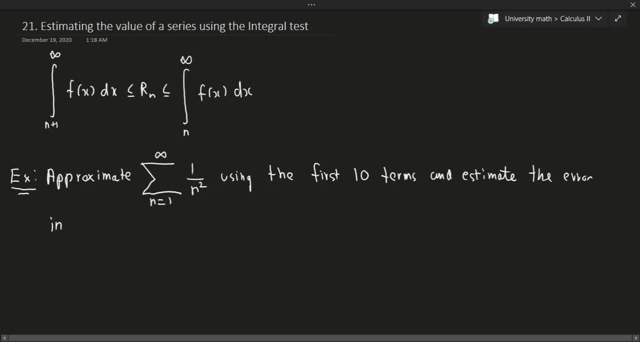 in this approximation. Okay, before we move on, this thing actually has a value. This is known as the Bessel series, which was actually very cleverly found by Euler back in the day, And this is actually equal to pi squared over 6.. 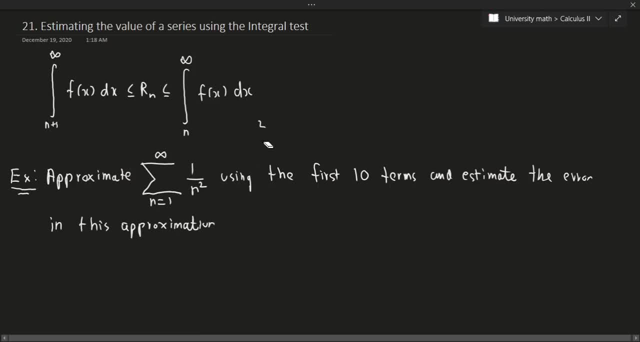 The derivation of this is kind of complicated so I'm not going to cover it in this video, But you can Google this. You'll find lots of proofs online And I might even do a video on this later if I feel like it later. 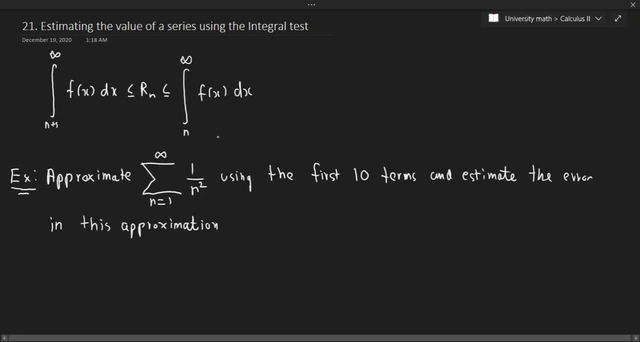 But, that being said, we can use that kind of benchmark to figure out how, approximately how close this approximation is. So pi squared over 6 is approximately, I believe, 1.6 something. So I'm just going to go ahead and calculate that out real quickly. 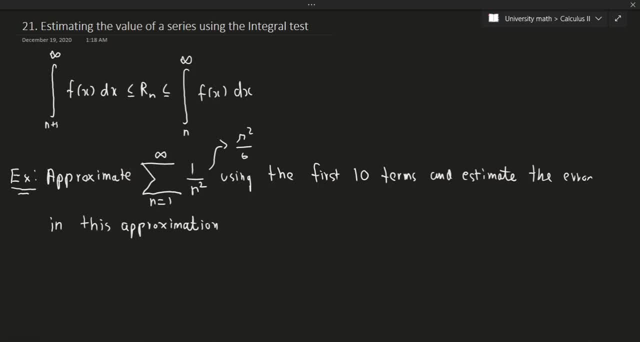 to make sure that this is at least somewhat close to my approximation. So this is approximately 1.64493 to 5 decimal places. So let's go ahead and talk about how to you know, use this. So approximate this thing using the first 10 terms. 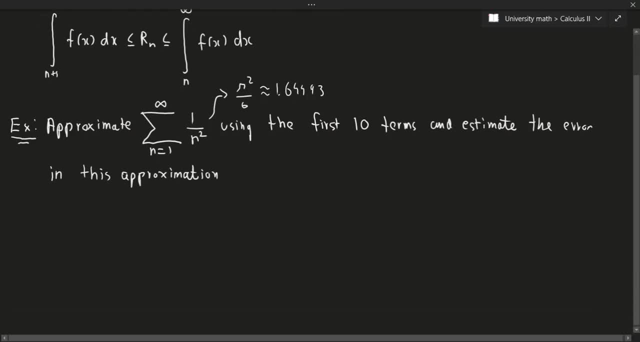 Okay, so we will quite literally sum up the first 10 terms. So for n equals 1, we get 1 over 1.. Then 1 over 2 squared, Then 1 over 3 squared, Plus 1 over 4 squared. 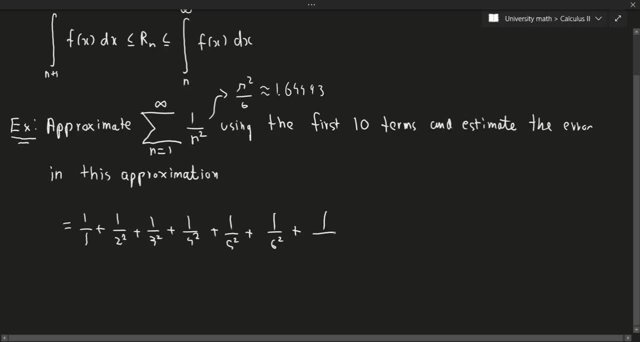 1 over 5 squared, 1 over 6 squared, 1 over 7 squared, 1 over 8 squared, Plus 1 over 9 squared, Plus 1 over 10 squared. So this will be the summation of the first 10 terms. 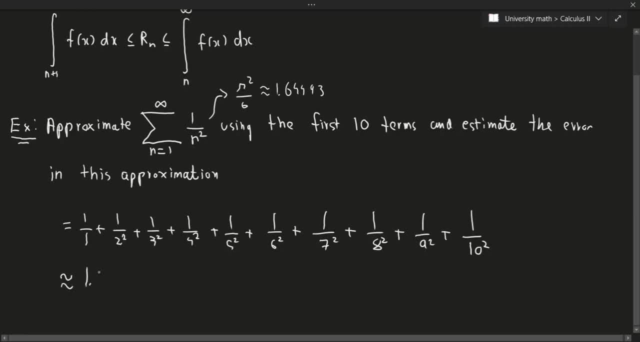 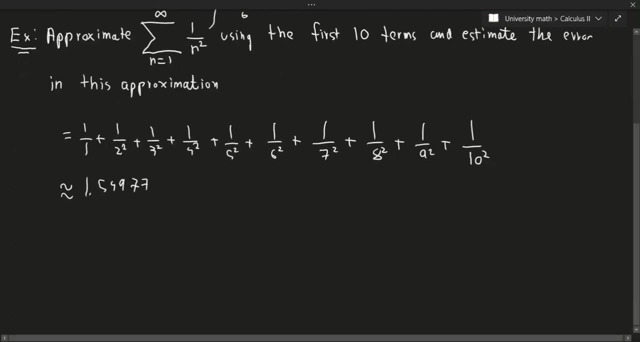 As you sum this all up, you'll get about 1.54977, etc. And we'll just truncate it right there. actually, Now, how bad is this error? So what is the error in this approximation? So, according to the integral test, 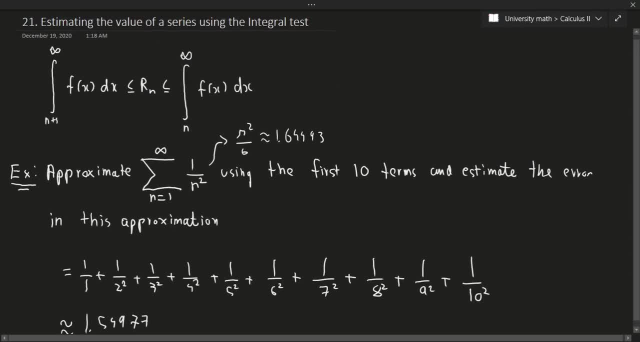 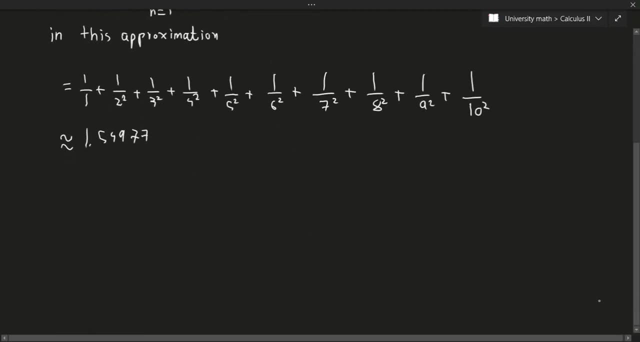 whatever error we have left over by using the next term in the series will always be less than or equal to this particular integral. Okay, so let's just take the integral of this thing. So recall, our integral was 1 over n squared. 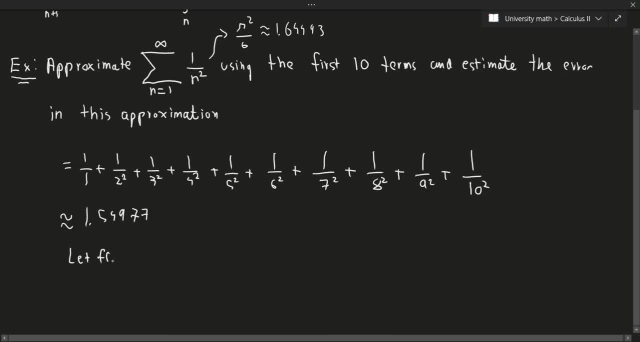 So let f of x be equal to 1 over x squared. So now we have the integral, from 1 to infinity, of 1 over x squared times dx. Okay, so if we take the integral, the integral of this thing, well, this is going to give us the limit. 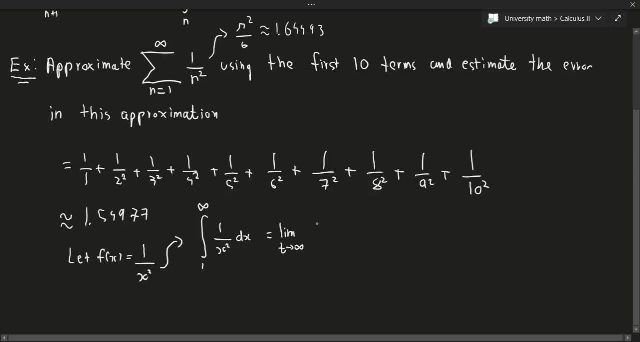 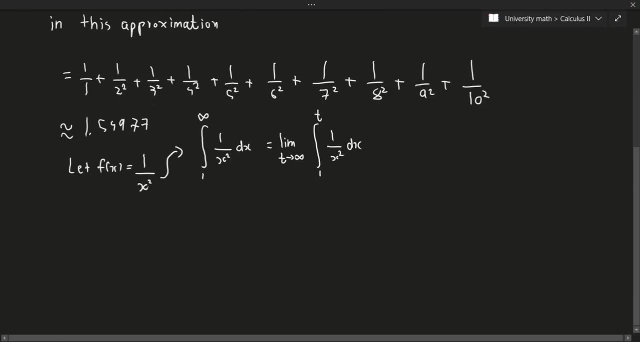 as t approaches, infinity of the integral from 1 to t, of 1 over x squared times dx. Okay, how does this help us? Well, what we can do now is I'll let you do the integral on your own, but if you go and do the integral, you get the limit as t goes to infinity. 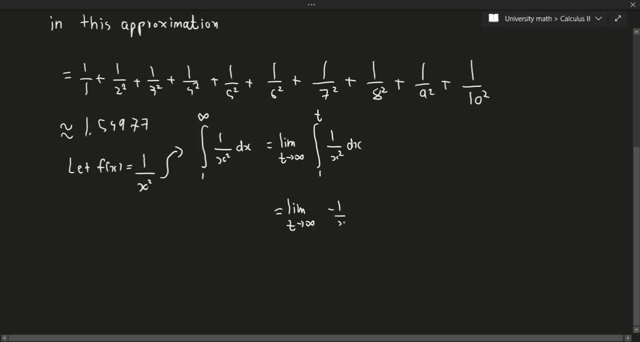 of minus 1 over x from n to t. And just to be very clear, the bounds are from n to t, not 1 to t. That was an accident, And the reason I'm picking n is because here we had an n. 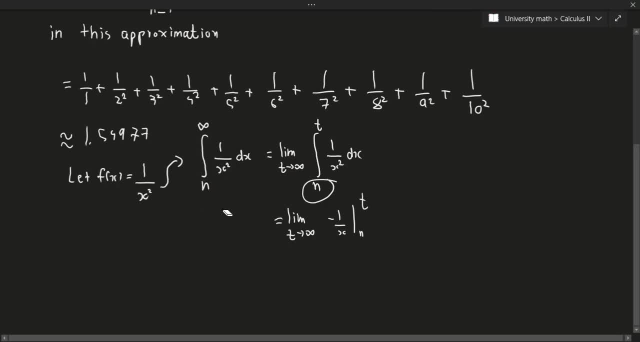 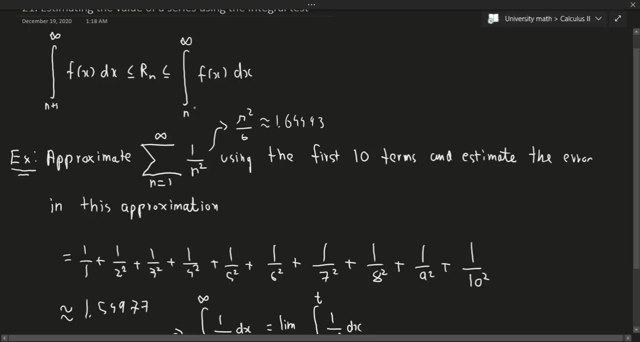 So that's why I'm using n as my lower bound right there. And the reason we're using n in the first place anyway, is because we're making sure that our remainder, or the error in our estimate, is less than or equal to whatever remainder we truncate at. 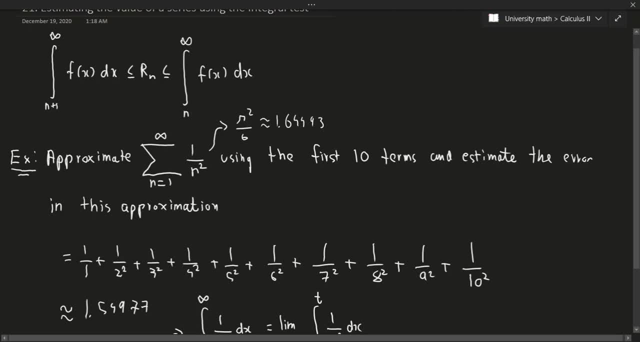 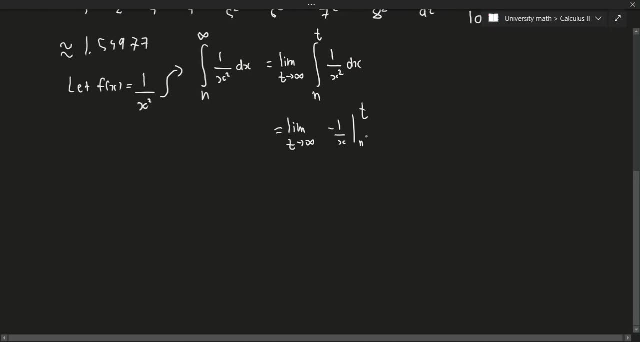 So in this case we are truncating at the nth value. So that's what we are integrating to. So we go from n to t. So in this case we get the limit, as t approaches infinity, of minus 1 over t, plus 1 over n. 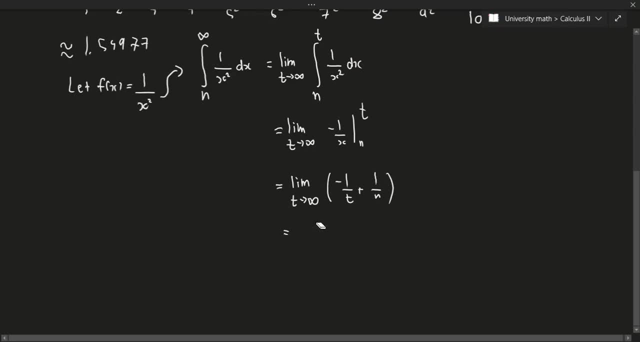 But then if you take the limit of this, it's the limit as t approaches infinity, so we're just going to get 0 plus 1 over n or 1 over n. So let's take a look at this. 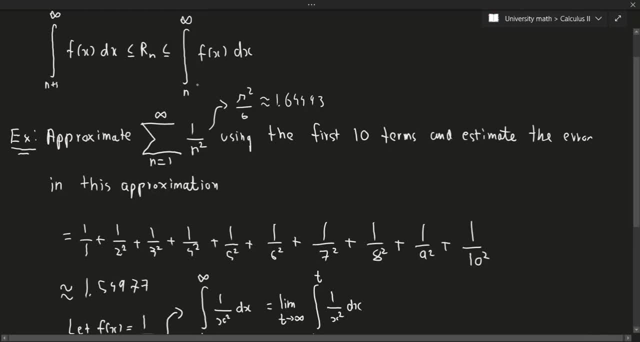 As I mentioned, the remainder is basically starting with n, and n is the number of terms we're using to sum up in this particular series. In this case, we're summing with the first 10 terms, So we just plug it in 10 there. 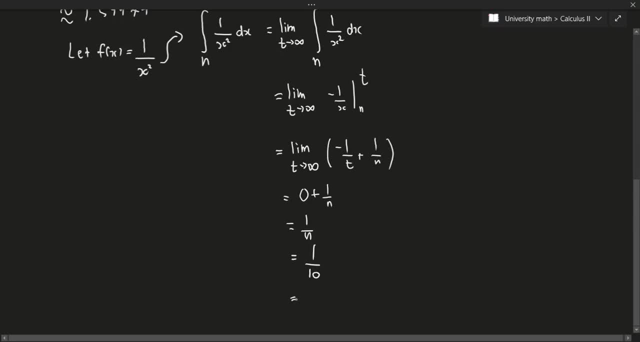 Meaning that the error in this estimate is 1 over 10, or 0.1% Or 0.1.. Or if you kind of divide this by 100, we're going to get 0.001.. I believe that's right. 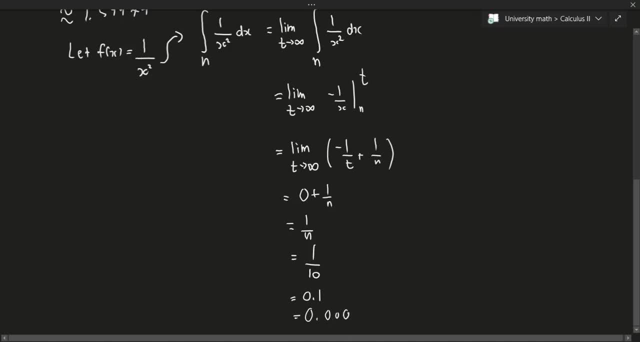 Yeah, cool, Yeah, okay, that's better And that will be the error. In fact, I'm also going to not. I'm also going to not, I'm also going to not. I'm not going to write this percentage. 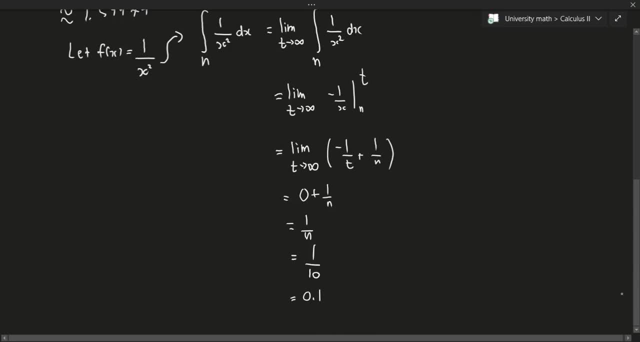 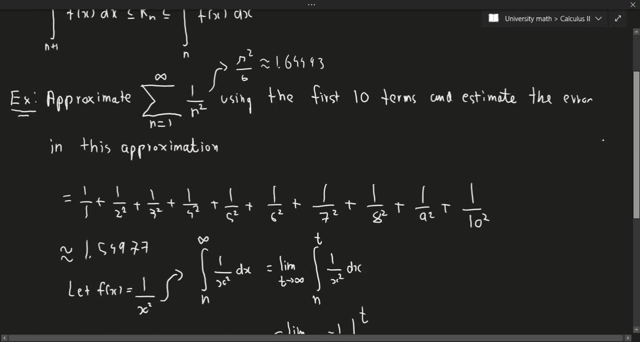 but I'm just going to write that as a decimal. But my point is that the error is going to be about 0.1.. That's really good. That's not bad at all. So let's kind of recap what we did here before we move on. 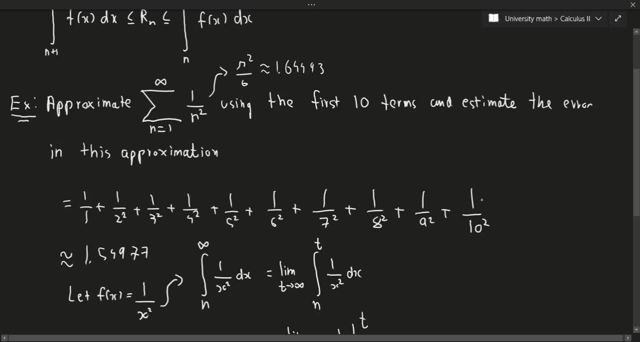 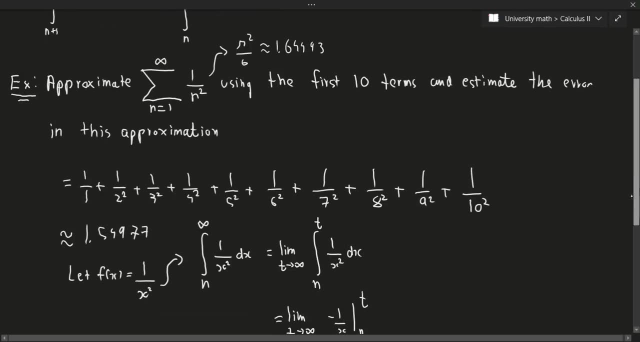 We were asked to use the first 10 terms to approximate the value of this series. Well, that's easy. We just literally added up the first 10 terms To find out how bad the error is. we used this particular test. So this is the integral test. 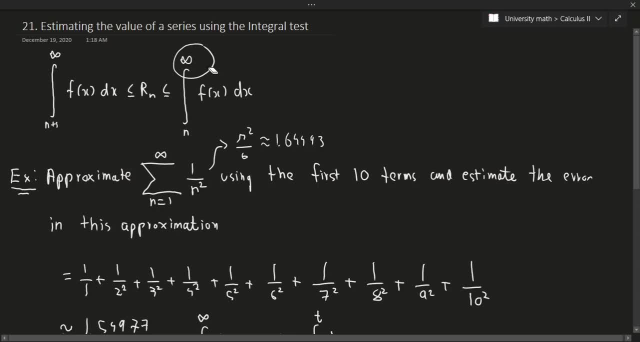 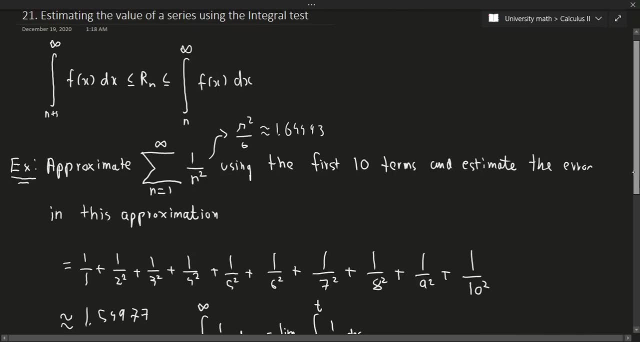 and then we integrate. We integrate from n equals 10, technically- to infinity, But we should probably. It's a good idea to leave it in terms of n, though, in case we need to use more terms to estimate the error. 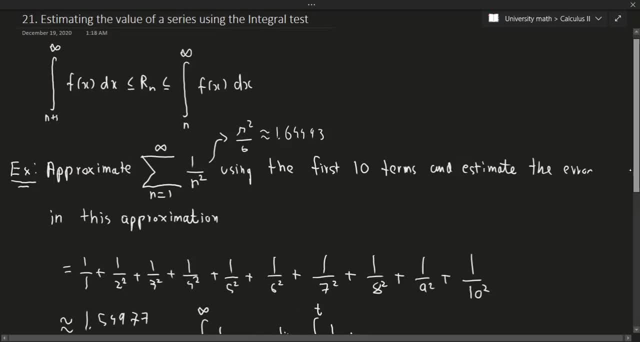 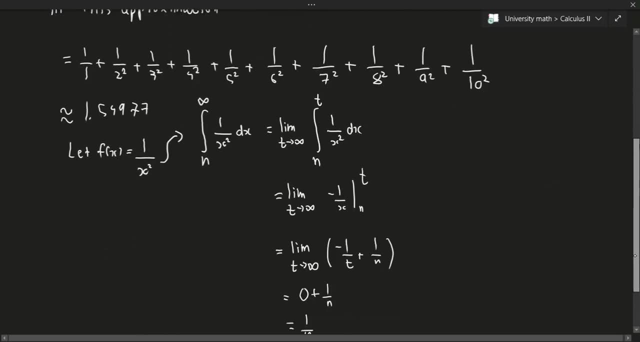 For example, 100 terms, 1,000 terms, 1 million terms and so on. So in any case, we integrate from n to infinity And after that we subbed in however many terms we summed up. So in this case it's 10 terms. 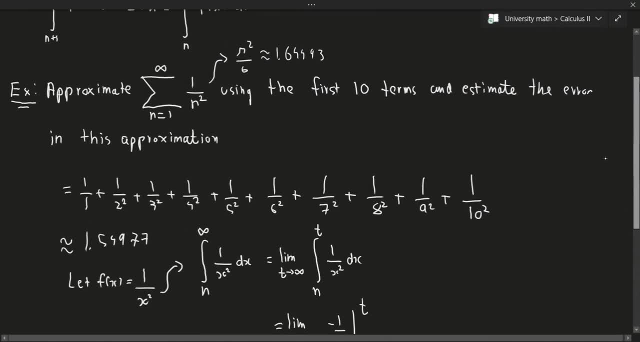 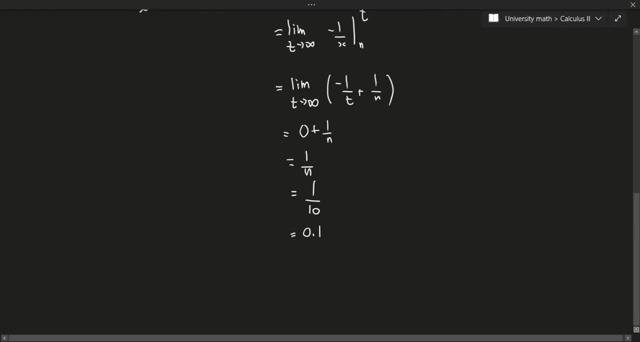 So we get an error of 0.1. And that is our error in this approximation. Okay, part B, This one is a bit more interesting. So how many terms do we need to add up so that? 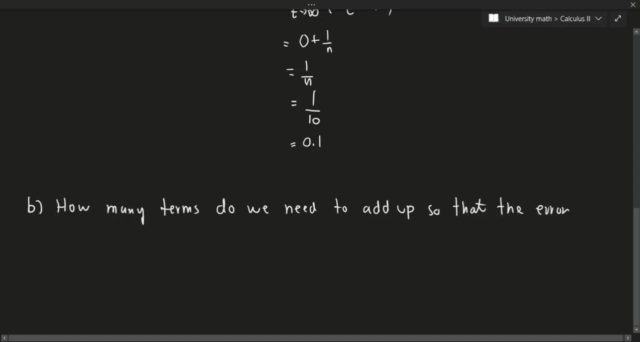 the error is accurate to 0.0001.. Now just to give you a sense of how accurate that is. that's pretty darn accurate. So we have to pick our n value so that our remainder or our error. 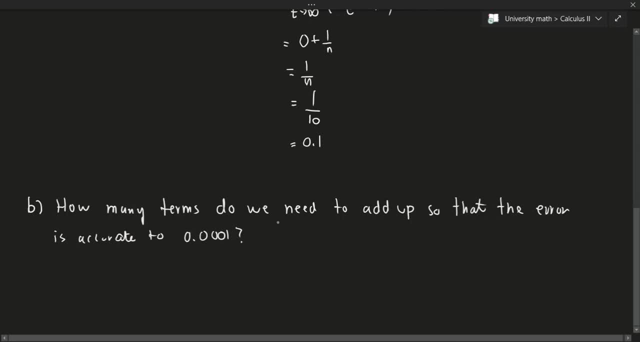 is accurate to this very specific amount. So this is the reason I didn't integrate from 10 to t, And the reason for that is because essentially, this thing has to be less than 0.0001.. Because that right there. 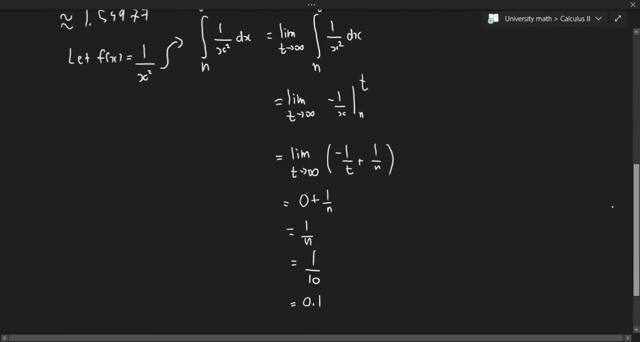 is the remainder in general, And we want to make sure that whatever we use for our remainder, it's always accurate to it in a certain range. So this is the reason I didn't use 10 as my lower amount. 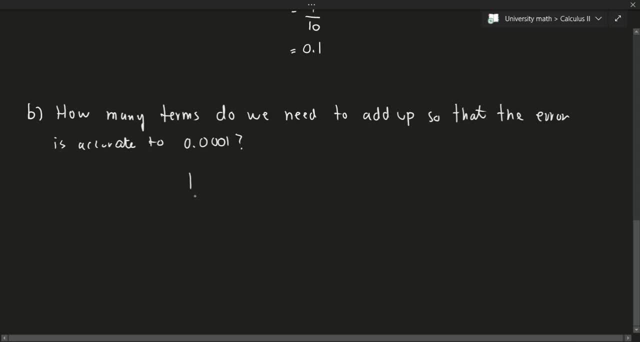 So what am I really saying here? I'm essentially saying that 1 over n, in this case, has to be less than 0.0001.. So what's really going on here? I'm saying that the remainder or the error. 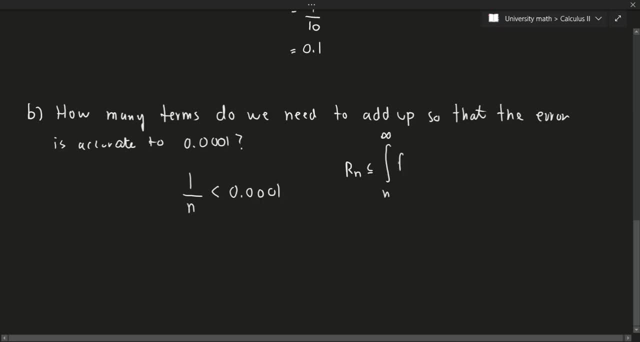 from n to infinity of f times, dx must always be true. This inequality always has to be true. So the remainder, in this case is always going to be accurate to this many decimal places. So here we just simply solve for n. 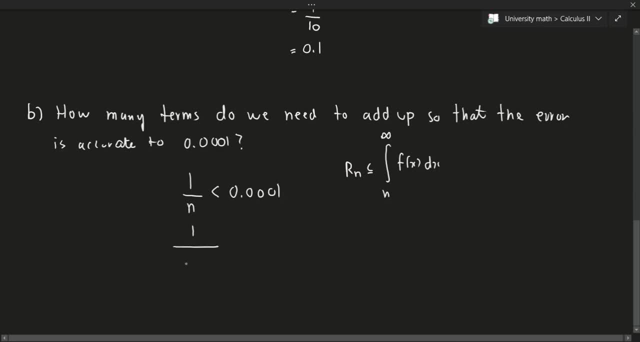 So that means we get 1 over 0.0001 is less than n. So we get n is bigger than 10 to the power of 4. Or 10,000.. Now we gotta be a bit careful. 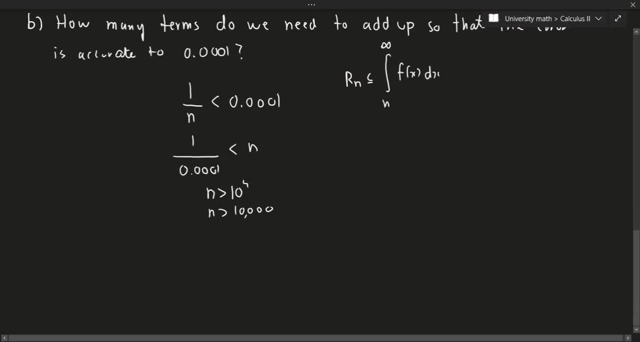 How many terms do we need to add up? So, because n has to be bigger than 10,000, and n is an integer, because we can't have half a term, we need at least 10,001 terms. as a result, 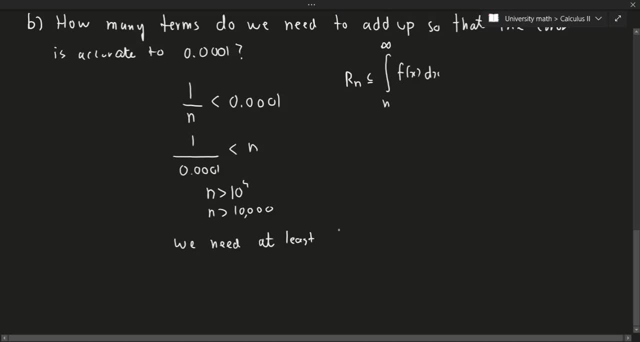 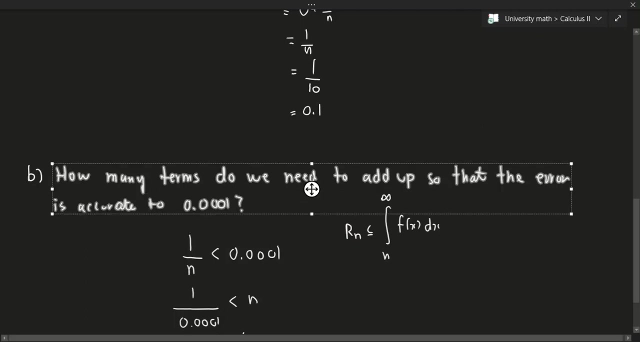 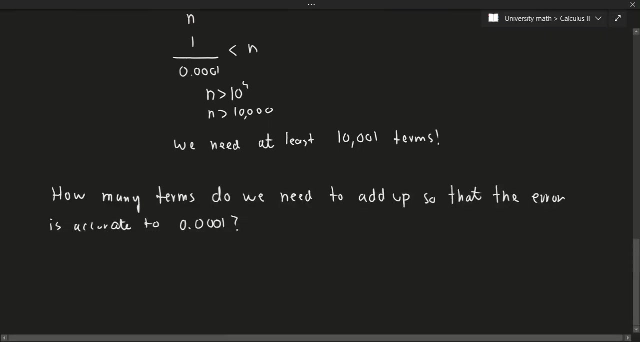 So we need at least 10,001 terms. Very interesting, Okay, Let's do another example of this thing. So Let me just copy-paste this question, because it's gonna be pretty much the same thing, Okay. 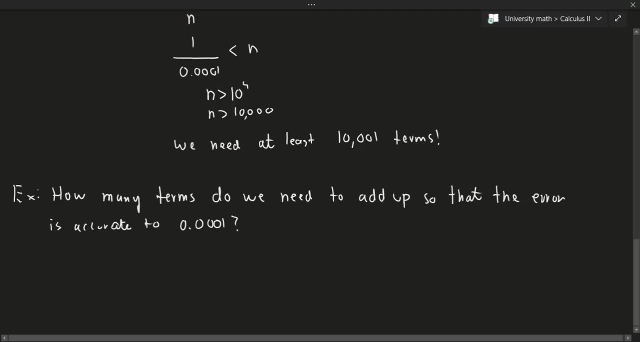 So how many terms do we need to add up so that the error is accurate to this time? it's 0.001.. And this time the sum in question is the summation from n equals 1 to infinity of 1 over n squared. 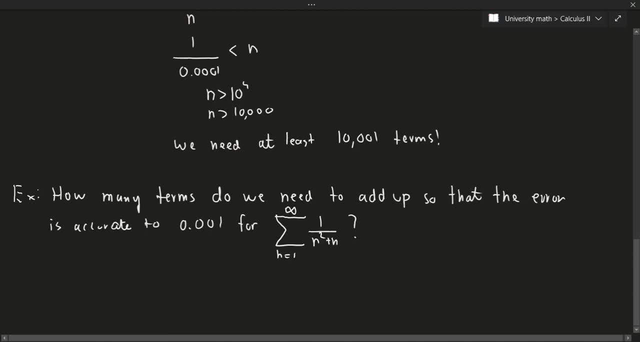 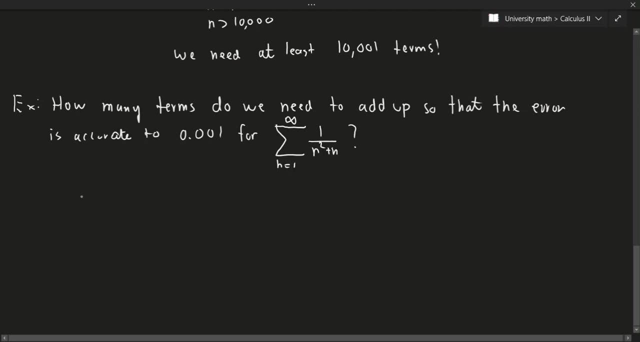 plus n. Okay, So how many terms do we need to add up to make sure that this is true? Okay, So once again, we're gonna be using the integral test on this thing, So we'll let f of x. 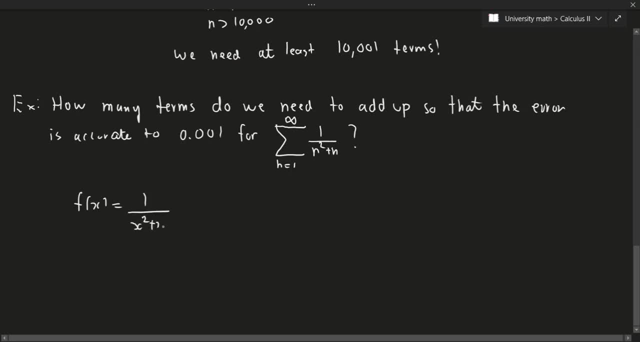 be equal to 1 over x squared plus x. So we're gonna be using partial fraction decomposition on this thing, because we're gonna be doing this. So, if you use partial fraction decomposition on this, which I'll leave you to the details, 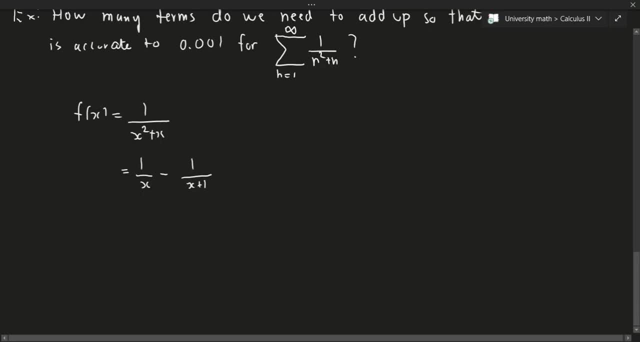 we're gonna get 1 over x minus 1 over x plus 1.. And now we get the limit, as t approaches infinity, of the integral from k, and we could use n- it doesn't really matter n to t of 1 over x. 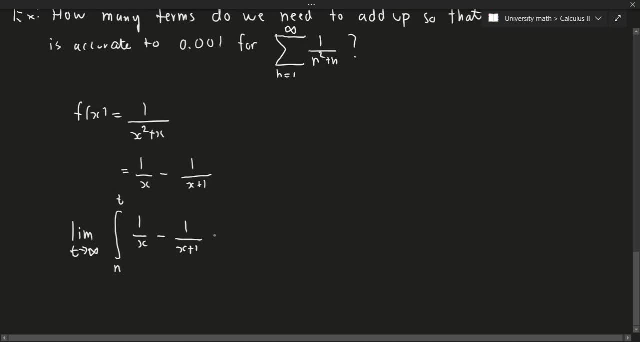 minus 1 over x plus 1 times dx. Okay, So now we can integrate both of these. So now we get the limit, as t approaches infinity, of the natural log of x minus the natural log of x plus 1 from n to t. 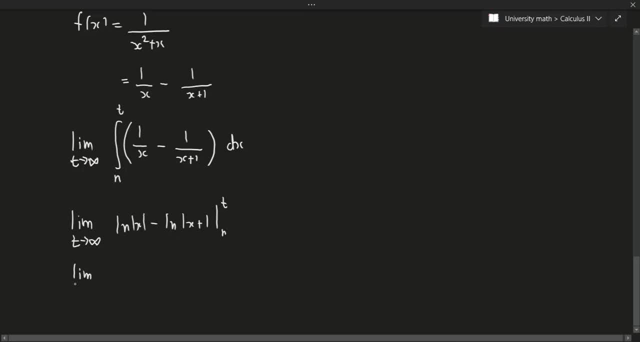 And if you go ahead and integrate this, we get the limit as t approaches infinity of the natural log of x over x plus 1 from n to t, And this is gonna give us the limit as t approaches infinity of the natural log of t over. 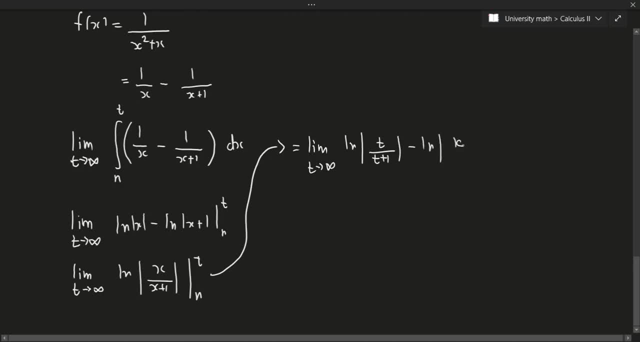 t plus 1, minus the natural log of n over n plus 1.. And then we can go ahead and do the limit on this thing. So this is just gonna go to well: 1.. And let's think about this. 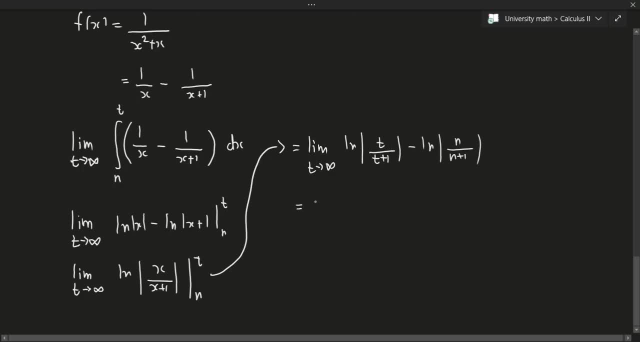 That thing is gonna go to 1, and natural log of 1 is 0, so that just disappears And this is just gonna stay as is And we can remove the absolute value because we assume that this integral is gonna be converging. 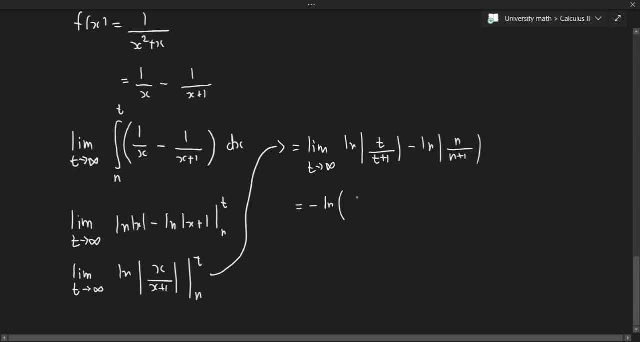 So we get negative natural log of n over n plus 1.. So I removed the absolute value because the reason that this is I'm making the assumption that this is that this thing is gonna converge, Because obviously I'm working with the assumption. 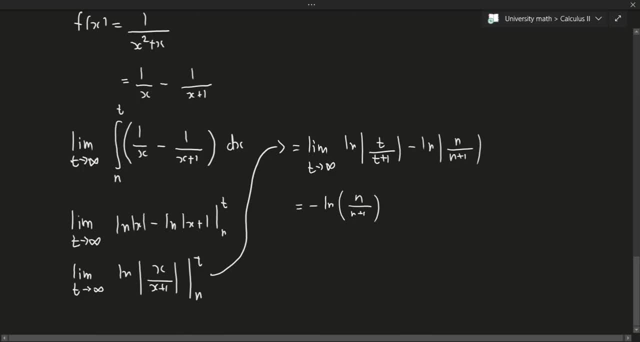 that this is gonna converge, Because if I take the limit of this to infinity by an integral test, this series is gonna converge. So you can check that for yourself. So it's safe to remove the absolute value. There's nothing wrong with that. 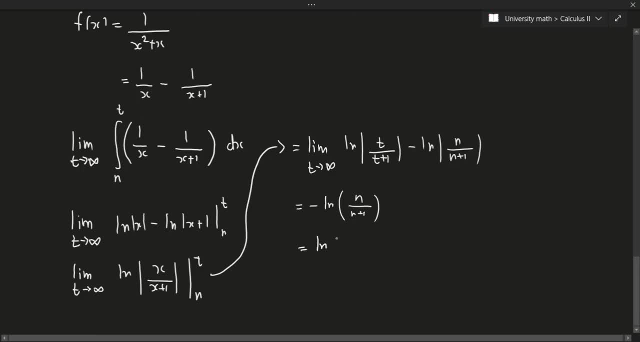 And then I can use the log laws So we can go natural log of n plus 1 over n. So that's gonna flip the fractions in the natural log. And let's take a look here. This has to be accurate.